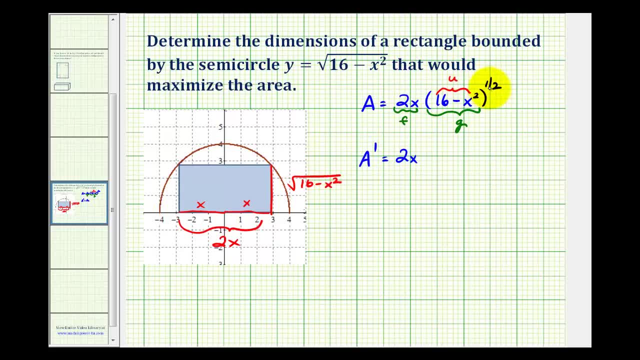 So we can think of this as u to the one-half. The derivative of u to the one-half with respect to x would be one-half times u to the negative one-half. but u is 16 minus x squared times u prime, which is negative 2x. 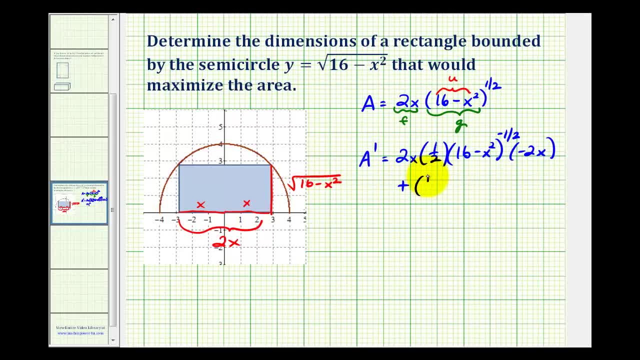 Plus the second function, 16 minus x, squared to the one-half times the derivative of the first function, which would be 2.. Now let's work on simplifying this. This 2 and this 2 would simplify out, So it looks like we'd have negative 2x squared. 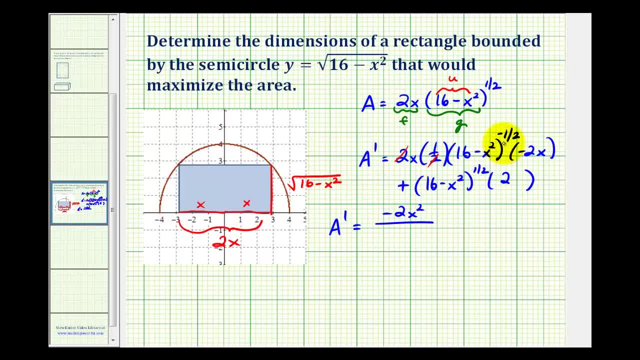 And then this has a negative exponent. so we'll move it down to the denominator. We'll have the quantity 16 minus x squared to the one-half Plus. here we're just going to have 2 times the quantity 16 minus x squared. 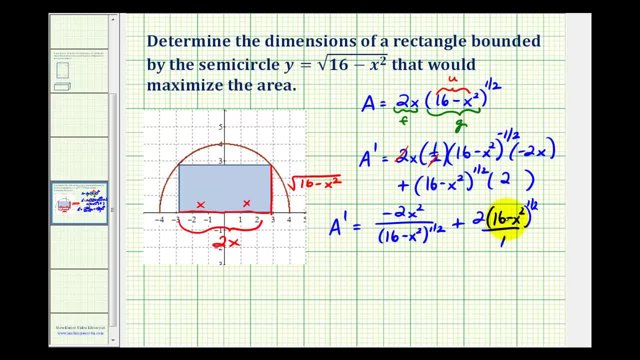 to the one-half. We'll go ahead and put this over 1, because what we're going to do now is combine these two fractions. We're going to do that by multiplying by the least common denominator, which would be the quantity 16 minus x squared to the one-half. 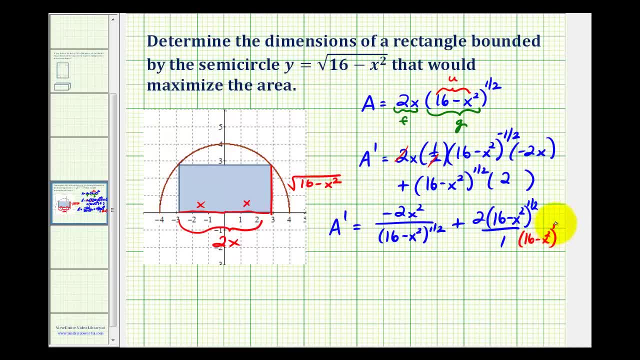 So multiply this fraction by 16 minus x, squared to the one-half over itself. When we do this, notice how we now have a common denominator. We have 16 minus x, squared to the one-half. in the denominator Our new numerator is going to be: 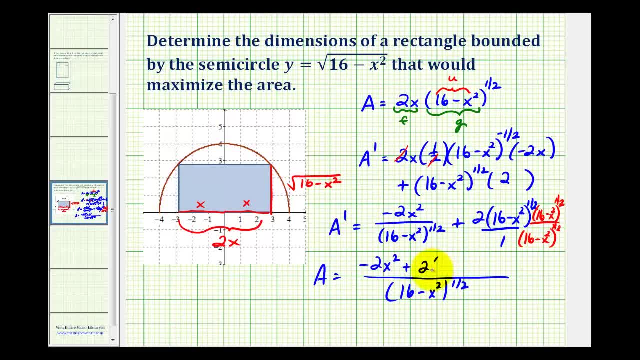 negative 2x squared plus 2 times. Now these bases are the same, so we'll add the exponents. We'll just have the quantity 16 minus x squared to the first, And now we can distribute here and combine like terms. 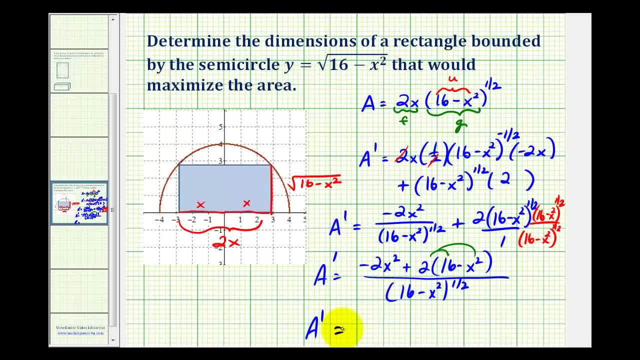 Oops, this is a prime. So a prime is going to be equal to: Here we have negative 2x squared, And then another negative 2x squared. That'll be minus 4x squared plus 32.. All over our denominator. 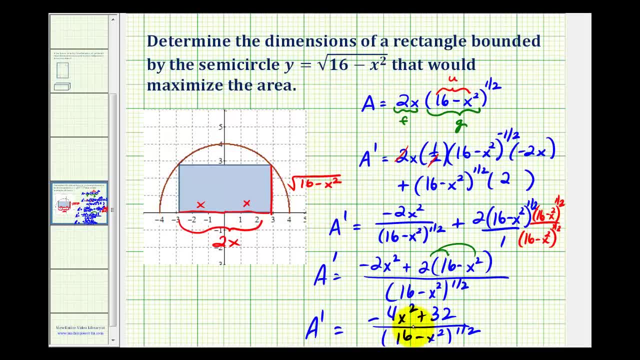 Now we want to know where the derivative does not exist or where it's equal to 0.. Now, looking at the denominator, we can see it's not going to exist when x is equal to 4.. If x is equal to 4,. 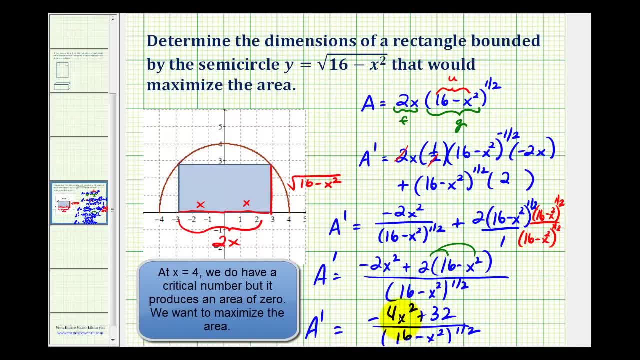 the height of the rectangle would be 0. So we can disregard that and only determine where this is equal to 0. And this is only going to equal 0 when the numerator is equal to 0. So if we set the numerator equal to 0, 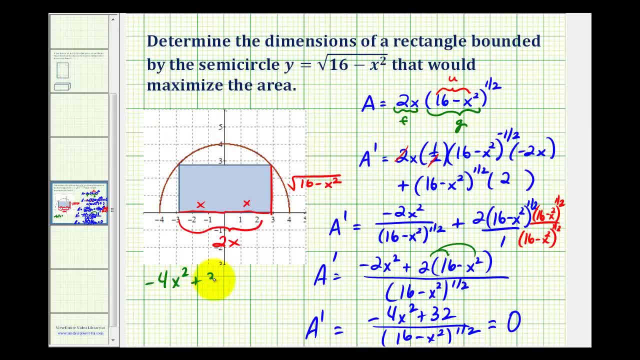 and try to solve. Let's factor out negative 4.. We're left with x squared minus 8 equals 0. So this will equal 0 when x squared equals 8. So we can take the square root of both sides. The two critical numbers are: x equals plus or minus 2, square root 2.. 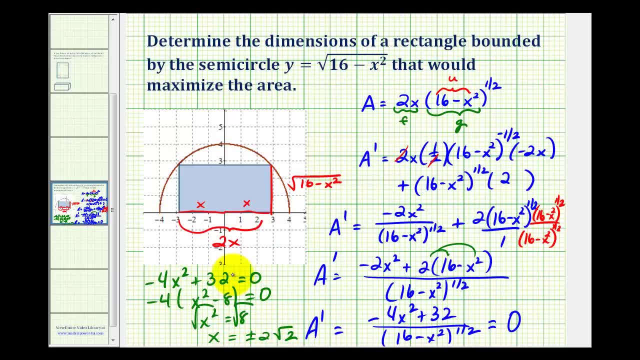 So these are the two critical numbers. But because one of the sides has a length of 2x, we know x can't be negative, Otherwise that would produce a negative area. So the only critical number that we have is x equals 2 square root 2.. 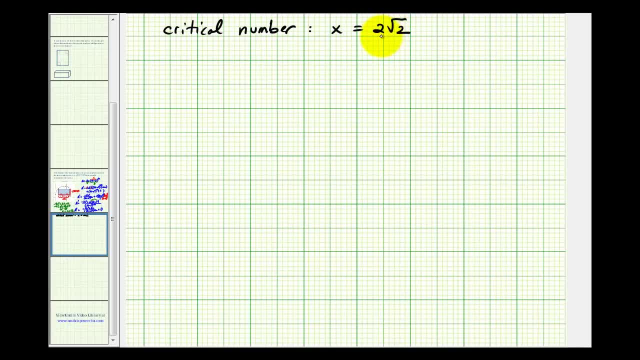 So this means that at this x value there may be a maximum or minimum function value which does represent our area. There's a couple ways of doing that. We could either use the first derivative test or the second derivative test. But looking at our first derivative here. 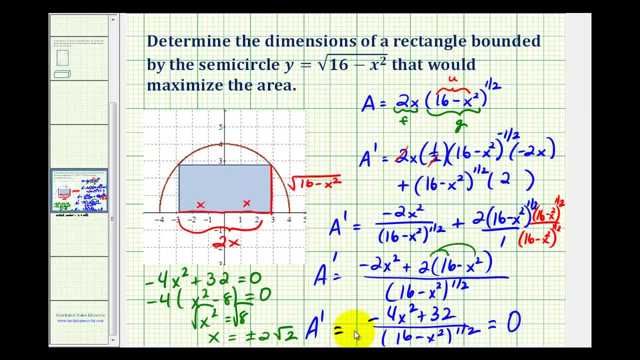 I really don't want to determine the second derivative of this because it would take some time. So for this example, I think we'll just look at it graphically. But what we're hoping to determine is: to the left of 2 square root 2,. 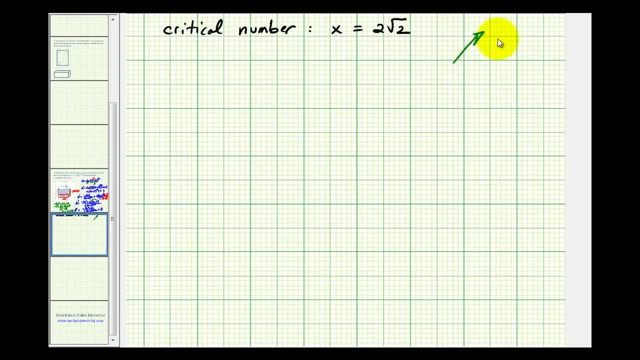 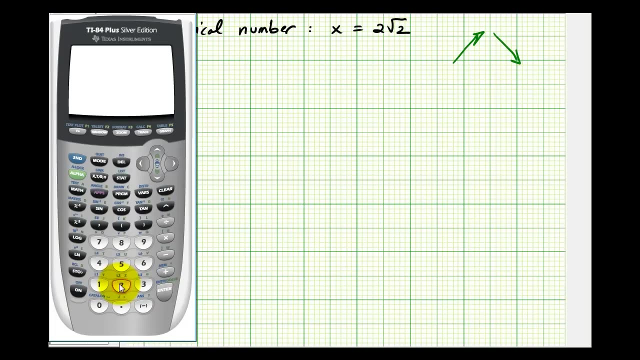 the function will be increasing And then to the right of 2 square root 2, we hope the function will be decreasing So that this verifies we'd have a relative maximum at x equals 2 square root 2.. Let's determine the decimal approximation for 2 square root 2.. 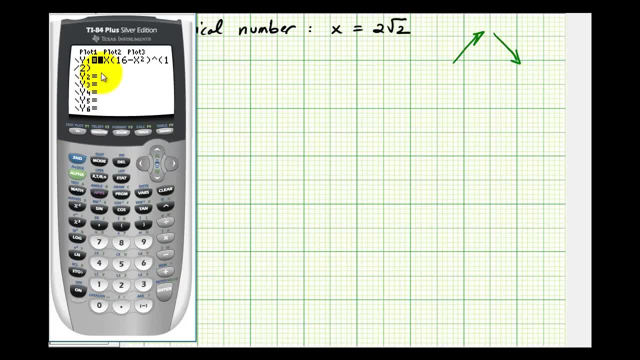 Approximately 2.8.. I've already entered in the original area function, So let's go ahead and take a look at the graph And notice: at about 2.8, right in here it does appear we have a relative maximum. 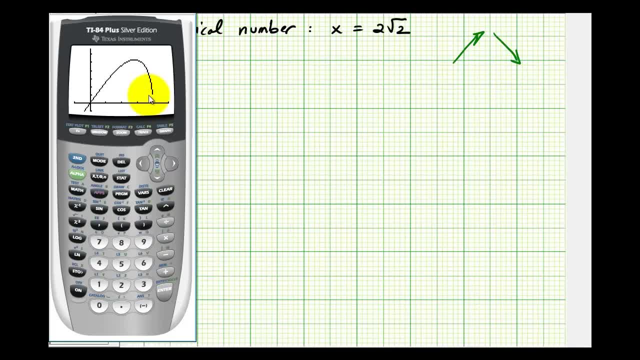 And the function is increasing and then decreasing. Therefore, we're going to go ahead and assume that at x equals 2 square root 2, we will have a relative maximum. So let's go ahead and determine the dimensions of this rectangle as well as the maximum area.